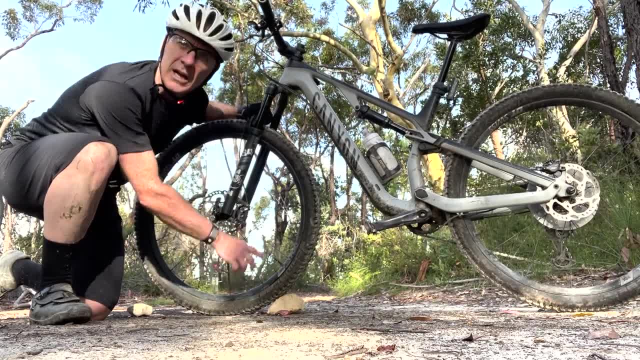 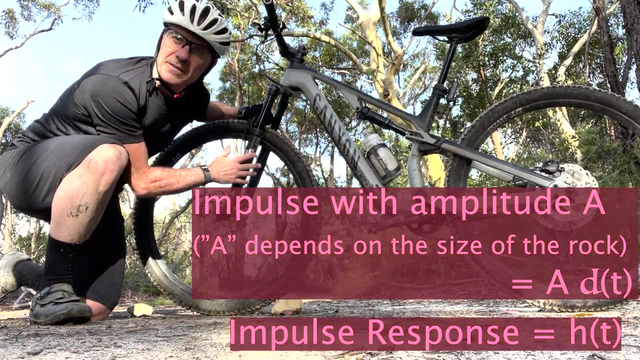 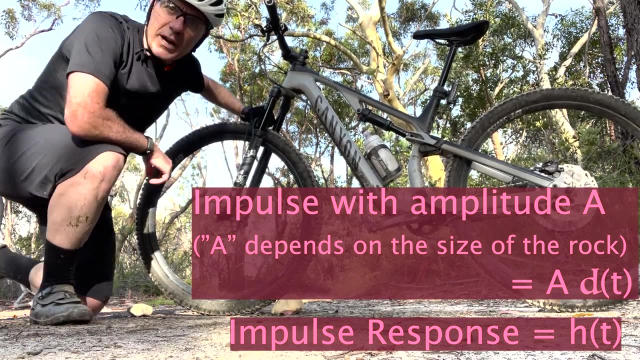 system, then we think of the rock as an impulse on the system. the forks have responded to the impulse. that's an impulse response and this has been the effect of the rock, of the impulse, on the system. Now let's think about what happens if there's another rock. so here's another rock, and if our forks 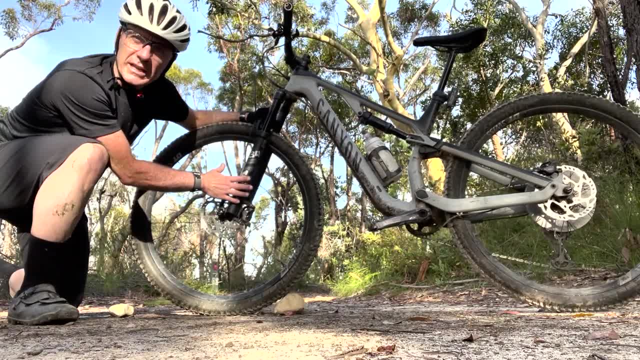 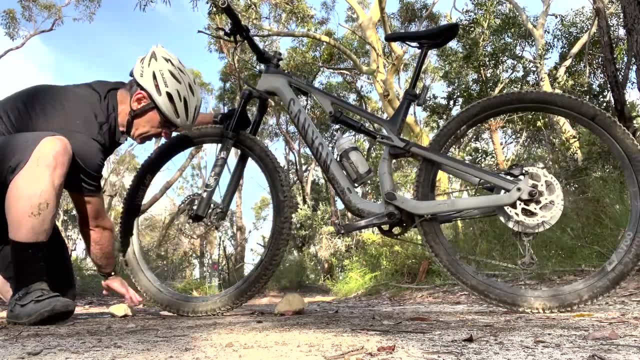 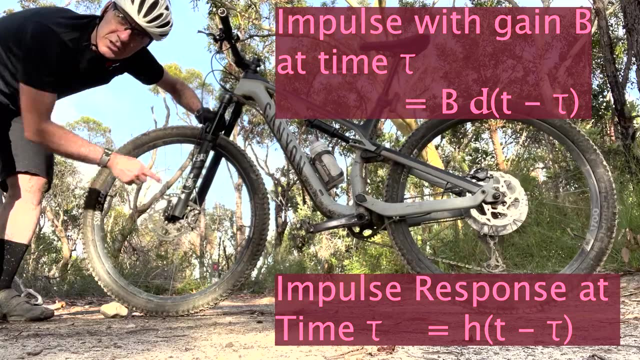 have responded to that system. so the compression in the forks has responded to that first rock and if it has returned to the steady state, when it hits the second rock, exactly the same thing will happen. so again, there will be an impulse, the forks will respond to the impulse, the forks will compress and then they will return to the steady. 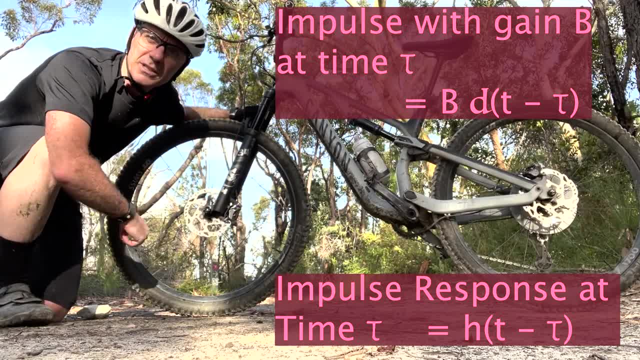 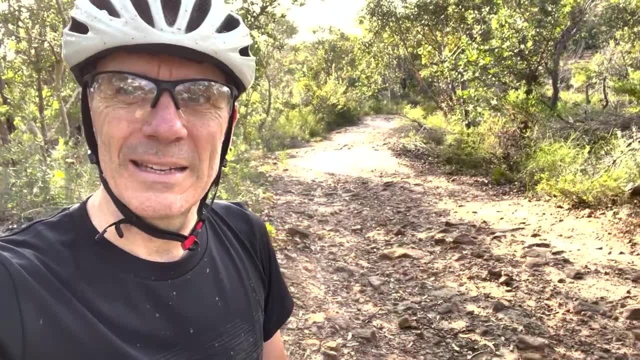 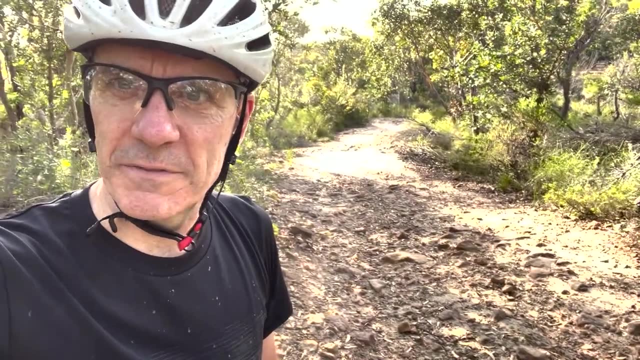 state. So this is when there are impulses acting on a system and where it has a chance to return to steady state. Now let's think of a situation where there are lots of rocks, like this path behind me here, and they're not spaced far enough apart for the system to fully. 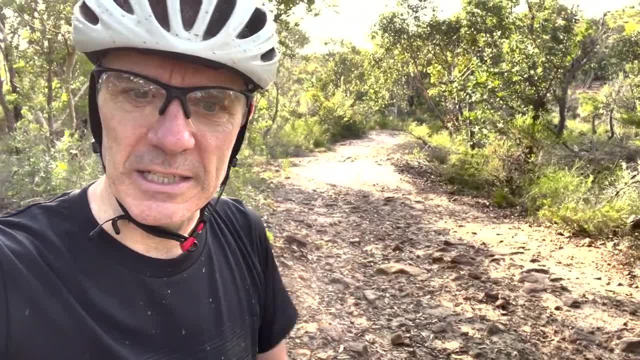 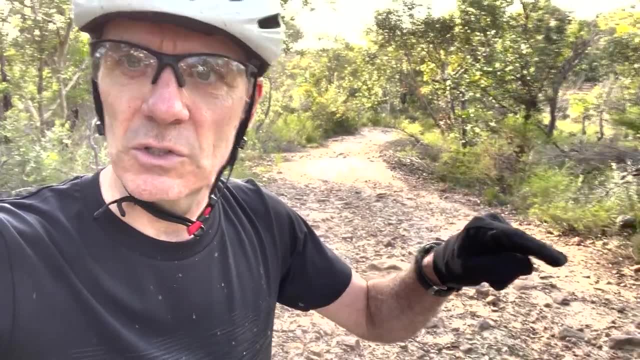 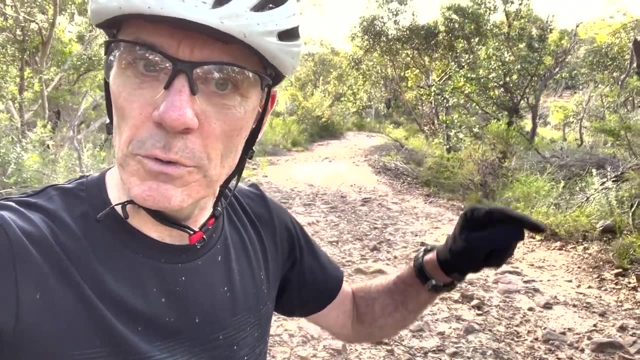 respond to the steady state, Then in that case there will be an initial response from the first rock and then it will recover and respond, trying to recover, to the steady state, but before it gets there, the second rock will also be an impulse, and so it will respond to the second rock. 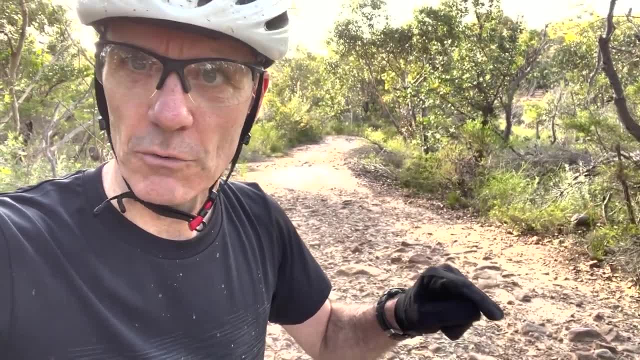 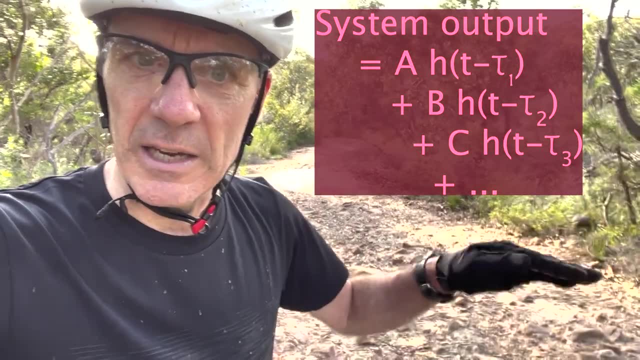 from a starting point, which is where it got to after the first rock, after its response from the first rock, and so on, And so each rock that it subsequently hits, it will respond to that rock and then start to return to the steady state. 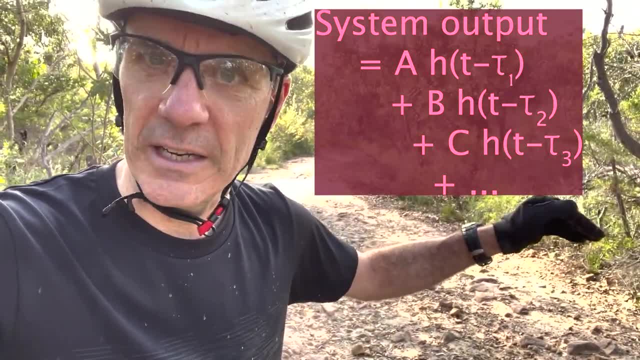 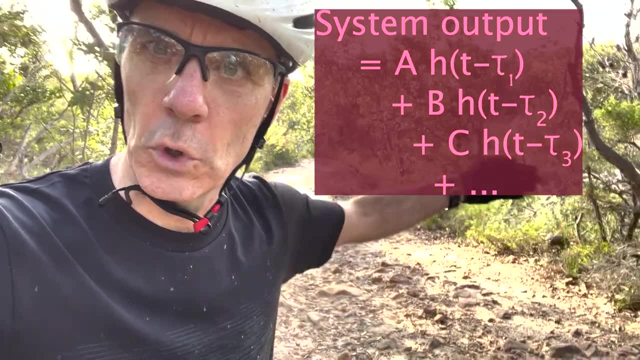 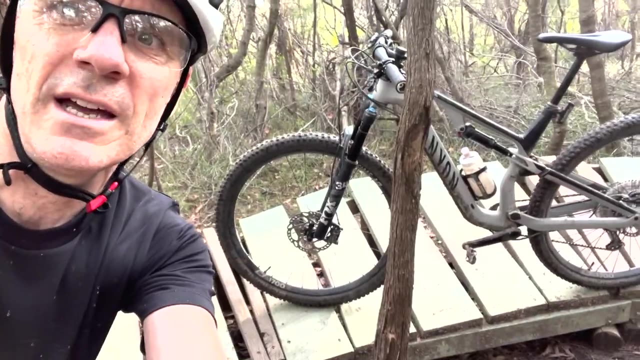 but then another rock comes, impulses again, and then it responds to that impulse and the accumulated effect of all of those impulses will give you an overall response to all of those impulses. So now let's think of this situation here where we've got a boardwalk. 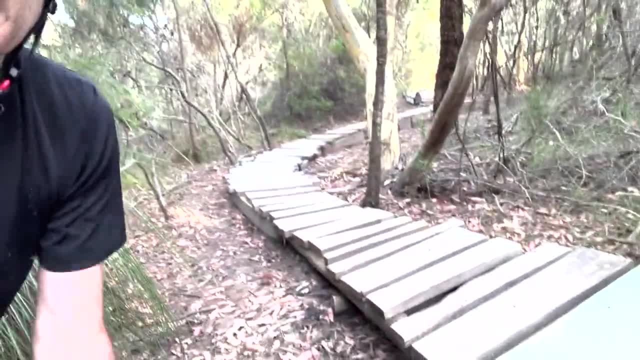 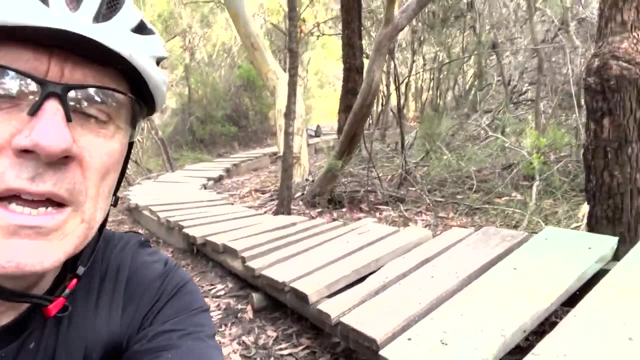 and let's think of each plank of wood as being an impulse, And they're now so close together that it's basically a smooth signal. So we can think of the boardwalk here. all these impulses so close together that they're a smooth signal.